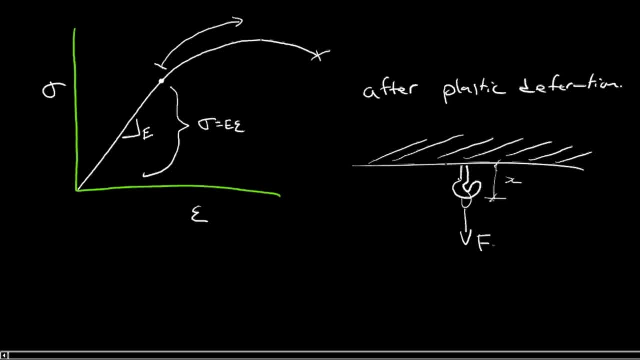 What's its distance, What's its length? Well, you can only, at this point, only do calculations if the force results in a stress that's less than the yield strength. If it's more than that, well, it's plastically deformed. 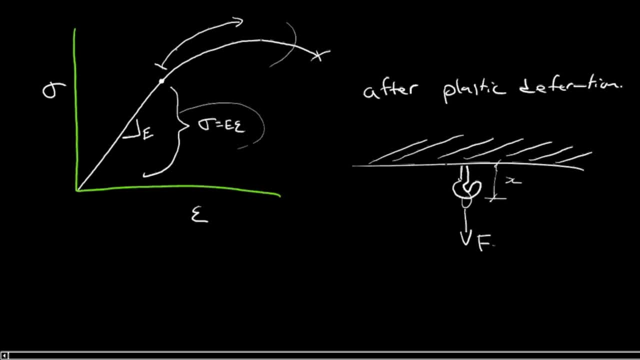 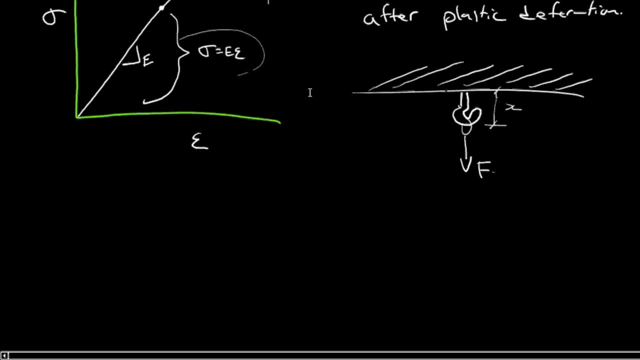 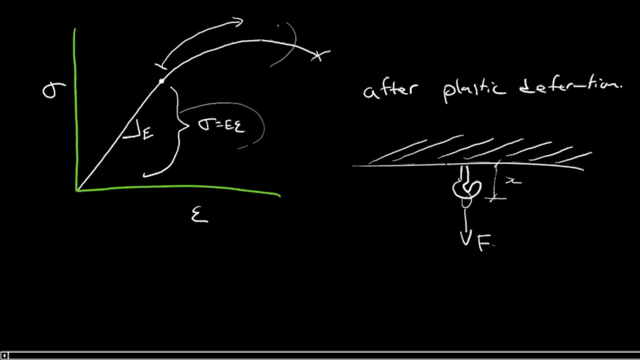 We couldn't deal with it unless we had some kind of way of describing the shape of the curve after it leaves, After it leaves the linear elastic region. And it's actually nice. We actually do have an equation that fits the curve, But we can't use engineering stress. 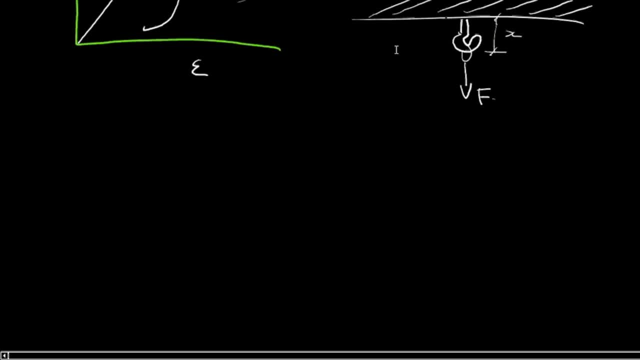 We have to use what's called true stress. So that's what I'd like to introduce for you right now. So, again, we're going to take a look at a generalized sample here. The idea, the goal is, of course, that we're going to go to be able to. 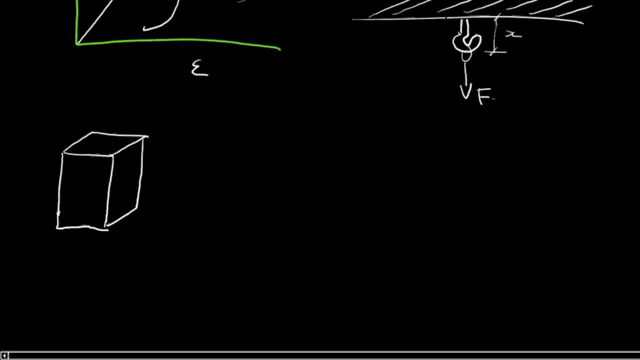 if you want to calculate and really understand plastic deformation. So there's our sample with its initial cross-sectional area, as we've discussed before And we said, well, when you load it it gets longer and gets narrower And it's that reduction in the cross-sectional area. 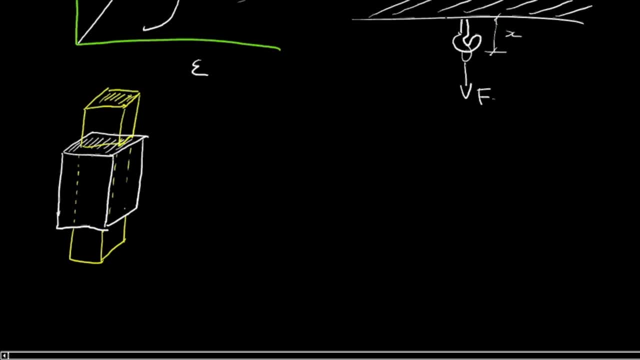 the deflection. And that's what we're interested in, Because this area- here now we could call it instantaneous area- Whereas this area, the white one, was the initial area. The initial area was what we started with, But then, while the load is applied, 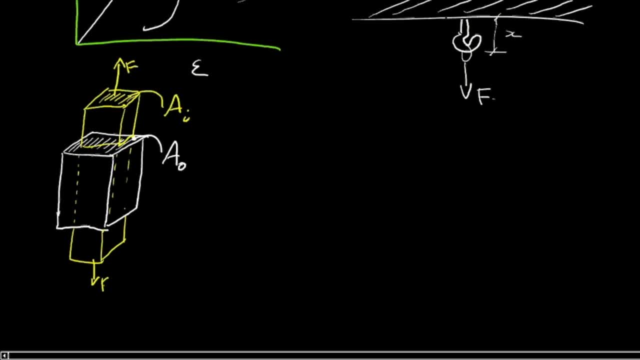 so sorry, let me draw the force in. While the load is applied, the cross-sectional area has decreased, So first thing we could do is we could say, all right, well, that means that this material itself is actually you know. 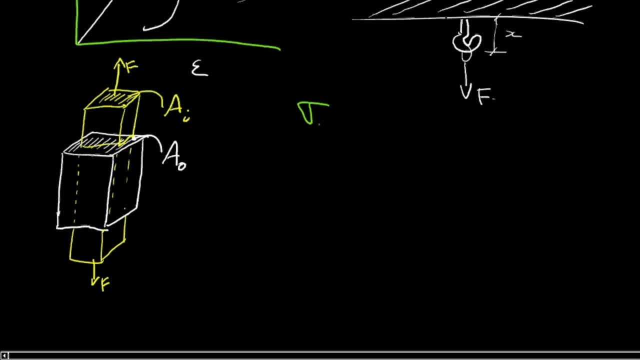 experiencing a force over a smaller area. So we could define the true stress as the force over that actual cross-sectional area. This is the true stress. This is the stress that the material itself is actually feeling And that subscript i is telling us. this is the instantaneous cross-sectional area. 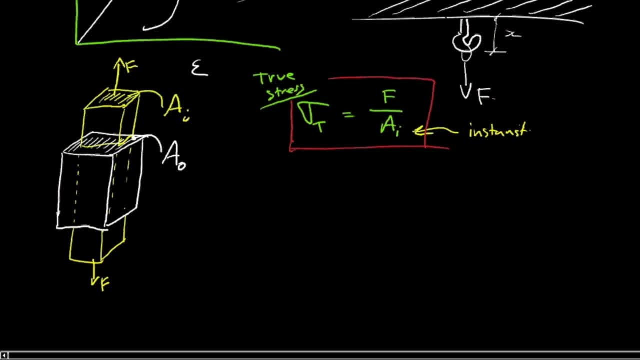 Instantaneous- I can't do more than one thing at the same time. apparently Instantaneous, I missed a? u- cross-sectional area. Instantaneous cross-sectional area, And I'll show you what the plot would look like in just a moment. 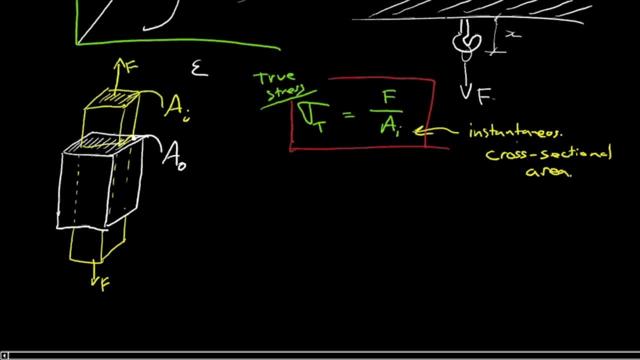 We could also do the same thing for the strain, although that's going to require a little bit more thinking. The true strain has to account for the fact that what we're doing is we're applying a change in length, right, We're elongating it over a certain length. 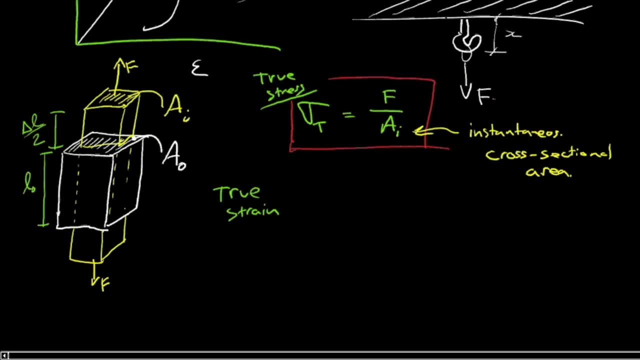 So the very first little bit of elongation is an elongation over l0.. But then After that the elongation is elongation over the previous length, which was l0 plus that little delta l. And so if you do that for infinitesimally small changes, 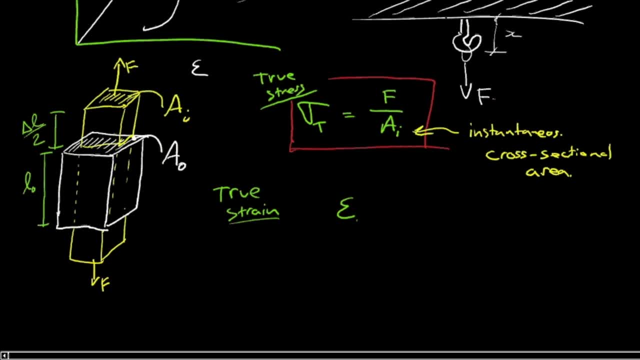 in length. the way we would write that is, we'd have to say OK. the true strain, what we're doing is we're integrating. We're integrating those infinitesimally small changes in length. that's dl by l. 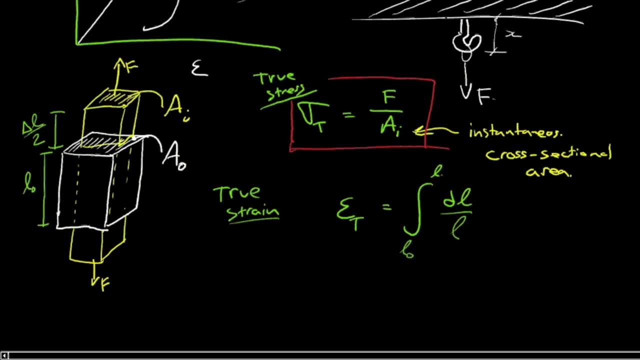 From l0, the initial length, to the instantaneous length. And so if we do that, we find that you have ln of l instantaneous minus 0.0,, which is ln of l instantaneous over l0.. OK, So we have. 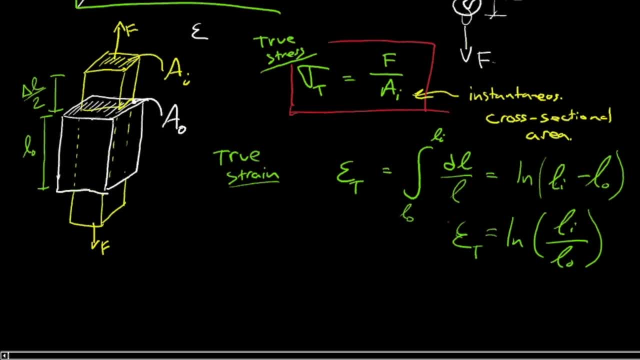 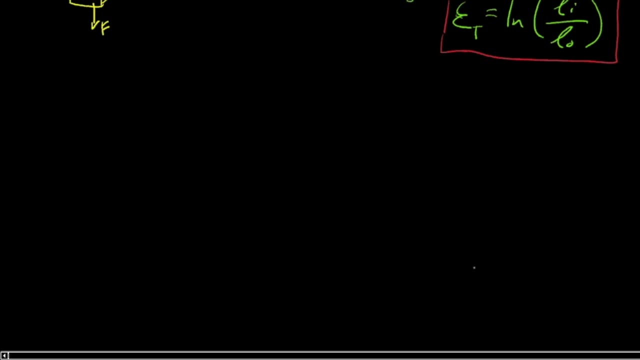 Another equation there and I'll put a box around that. So this is the true strain. OK, True strain. And if we take that true stress and plot it against the true strain, I'll show you what we'll get. Actually, let me just plot stress and strain. 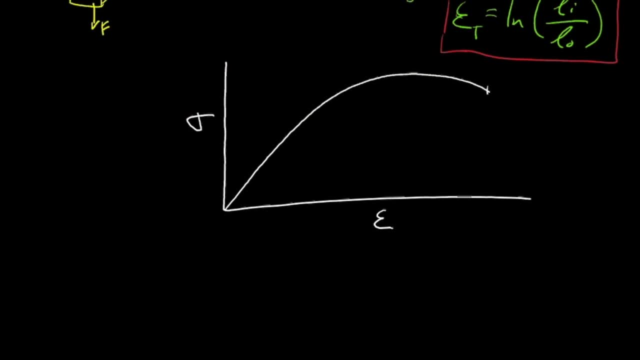 And I'll show you what we've already seen, That's the engineering stress-strain curve. And then what I'll do is I'll plot for you, After it starts to plastically deform, the true stress- So this one here continues to increase.